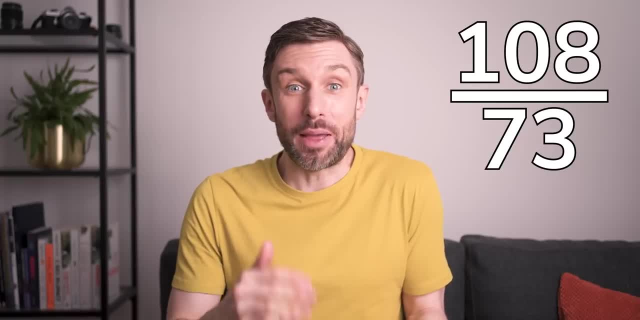 So the commonly quoted normal blood pressure is 120 over 80. So the commonly quoted normal blood pressure is 120 over 80. So the commonly quoted normal blood pressure is 120 over 80. Though some healthy people can measure a bit lower than that. 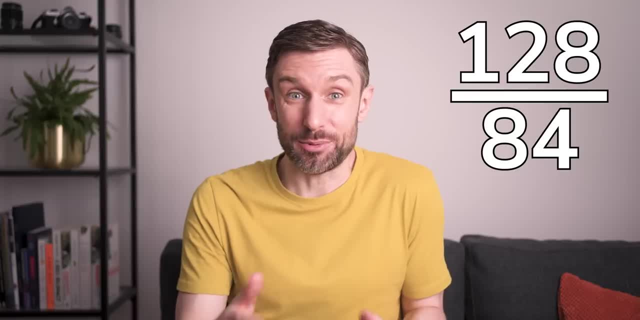 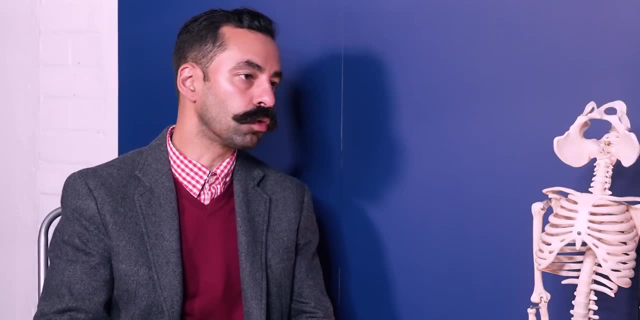 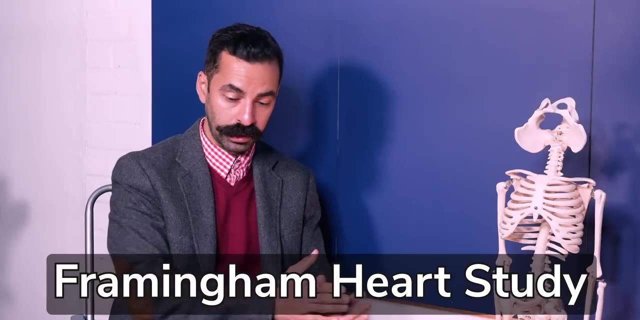 It's when blood pressure starts to creep above 120, over 80, that we run into problems. But why is high blood pressure bad for us? So blood pressure is an extremely important measurement and this comes out of Framingham landmark study in cardiology, a longitudinal study. 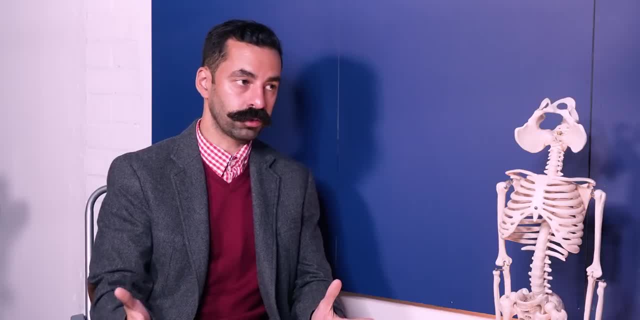 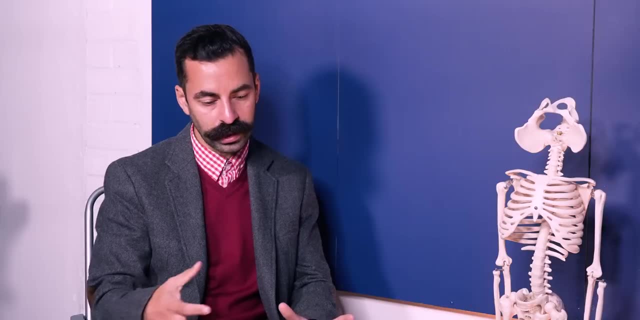 following up lots of people, And this is what identified a lot of the risk factors that we know about for heart disease, like high cholesterol and high blood pressure, emerges one of them, And the reason is is that high blood pressure reflects the fact. 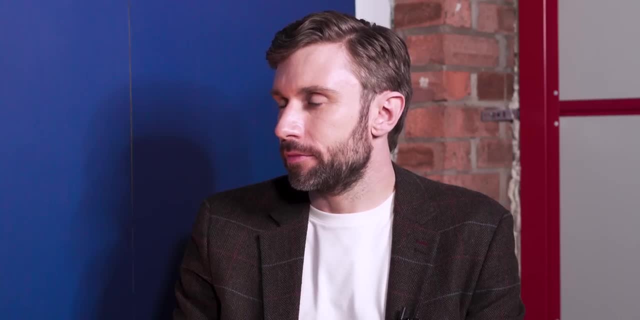 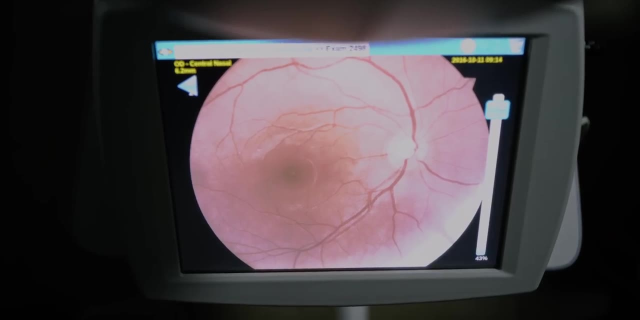 that your arteries are becoming less elastic, They're becoming stiff, And that's what happens as we get older, And this leads to kidney damage, heart damage, damage to your eyes. And what do these things have in common? Very small blood vessels. 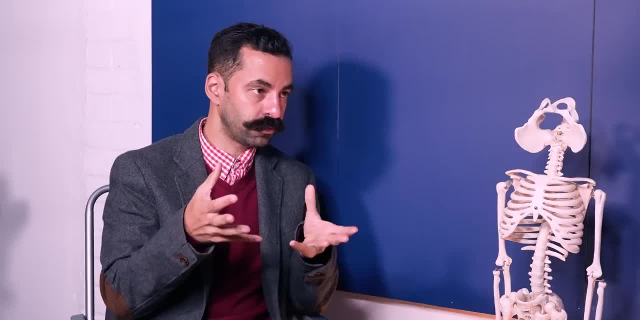 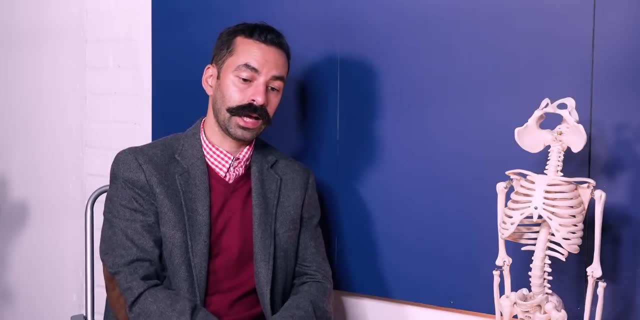 So it tends to you know, if you're having elevated pressure in vessels that aren't designed to handle this pressure, you're gonna get damage, You're gonna get little haemorrhage bleeding in these areas And these organs will start to fail eventually. The damage that high blood pressure causes is cumulative. Every year you live with it, more tiny blood vessels will break, And that's why it's never too early to start keeping an eye on your blood pressure and never too late to start trying to improve it. 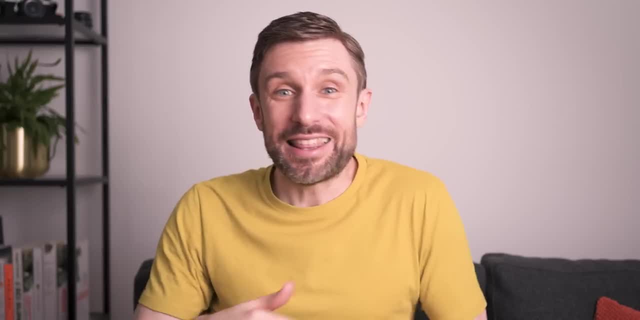 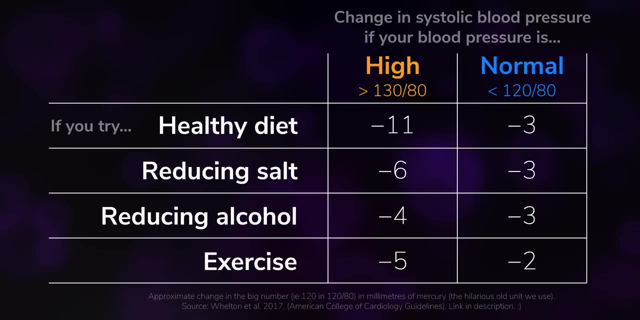 If you're regularly getting readings above 120, over 80, there's plenty you can try. Eating more fruit and veg, cutting back on salt and alcohol and getting more exercise are all great places to start, And if you're regularly getting readings, 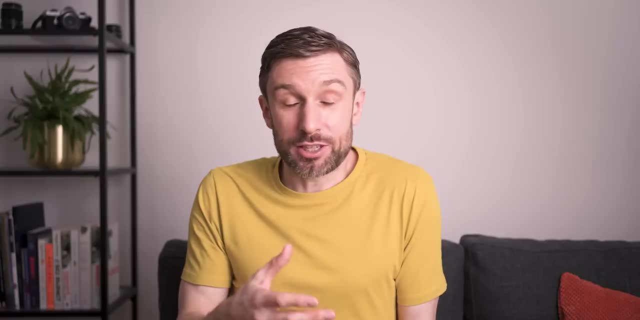 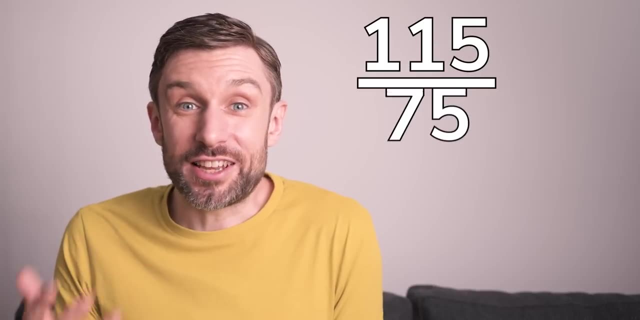 of 140 over 90 or more. it might be worth discussing this with your doctor, if they don't already know, and considering starting on medication Above 115 over 75, every 20 over 10 increase roughly doubles your risk of heart disease or stroke. 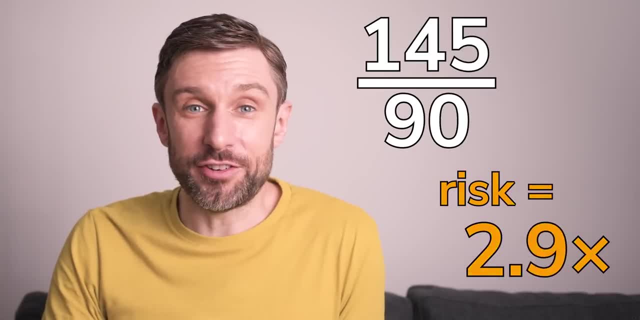 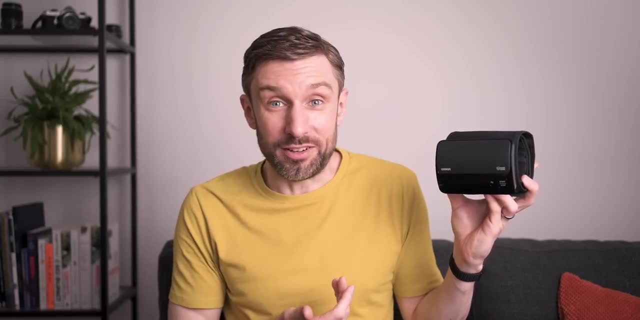 So 135 over 85 is twice the risk, 155 over 95 is four times the risk, and so on. So by making you aware of your numbers run a little bit high, this humble little device could save your life. And high blood pressure is a silent killer. 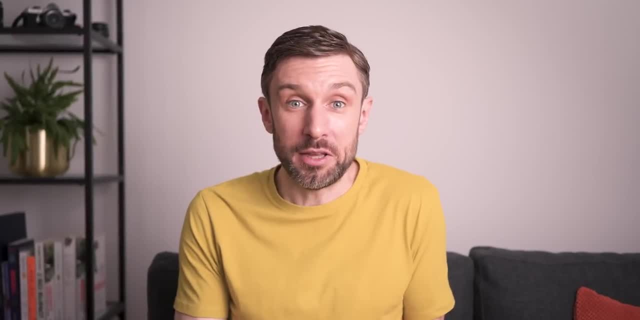 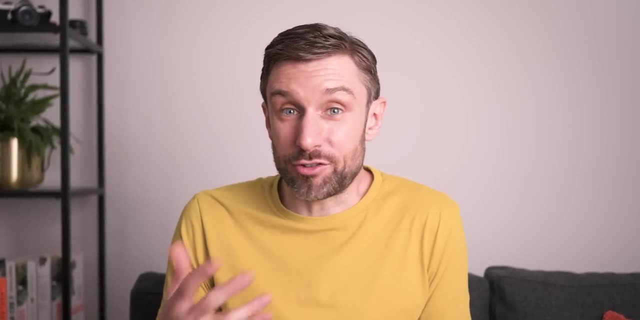 Globally, 40% of people over the age of 25 suffer from it, But the problem is it hasn't got any immediate symptoms. You can't feel if you've got high blood pressure, So that's why it's worth grabbing a blood pressure cuff. 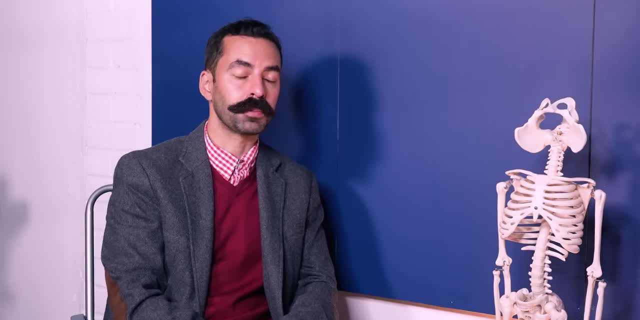 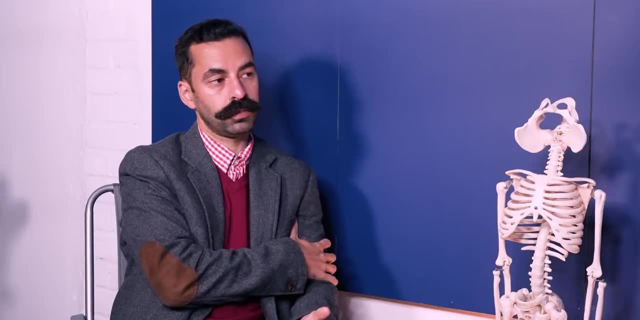 and seeing what's going on inside your circulatory system. The problem is is that measuring blood pressure is pretty hard And I'm sure everybody knows the way we normally do, that is with a cuff. If you have a cuff, that inflates and it's quite painful. it inflates because it has to go above the top number. It has to go above your blood pressure to then deflate. It's annoying. No one's going to tolerate having that being done all the time. So some devices have come out, sort of trying to measure this. 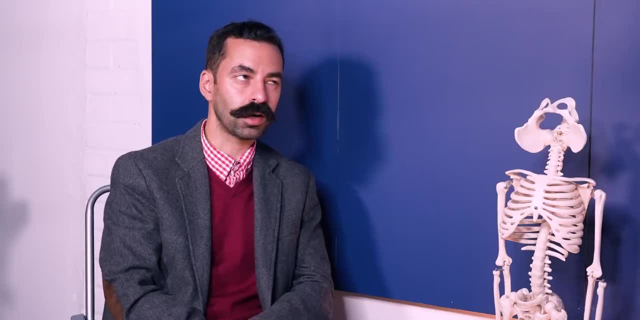 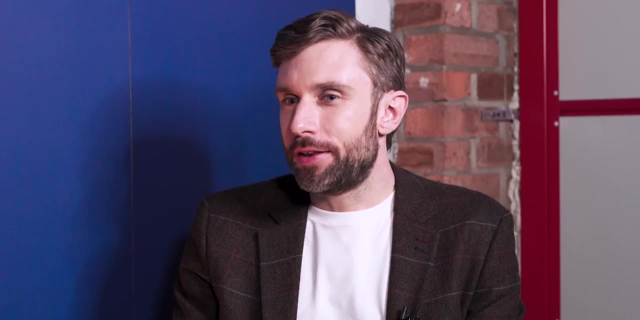 from the wrist in different ways and all kinds of different algorithms, But so far, to me it seems like the kind of holy grail. It's not, we're not there yet, And that's an interesting thing. It's an interesting question in terms. 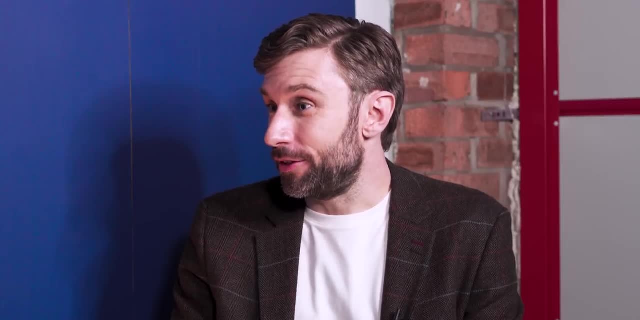 of the continuous monitoring as well, Because, again, if you look at the sort of clinical studies that have looked at this, this is again done in the doctor's office. There's this phenomenon: white coat hypertension. I suffer from terrible white coat hypertension. 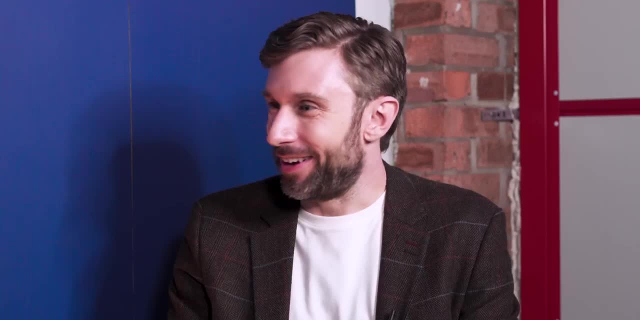 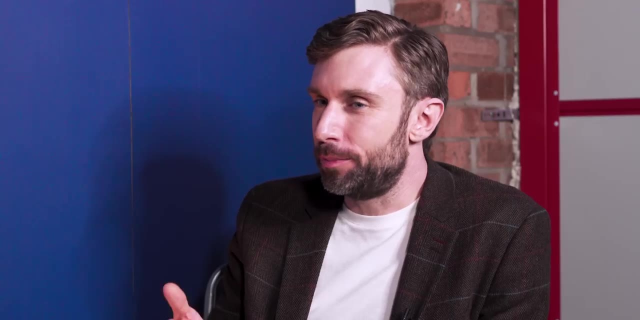 My heart rate and my blood pressure go right up. How are you feeling right now In the presence of a doctor? Terrible, Oh my God. And what's really interesting is comparing your blood pressure while you're exercising. So I've got a blood pressure cuff. 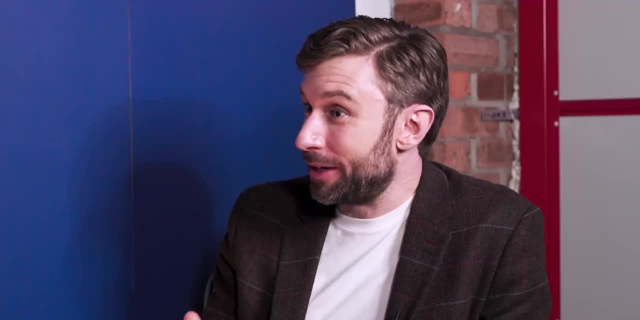 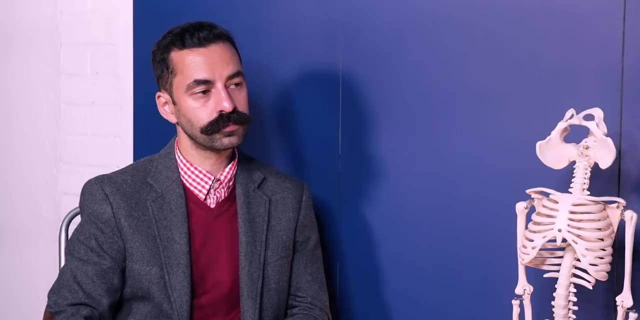 that I tried to wear while cycling And my systolic blood pressure. the big number was 160 something. Of course, that's probably normal, but I've just got no idea what these long-term measurements would actually mean. No, and we don't really have much data at all. 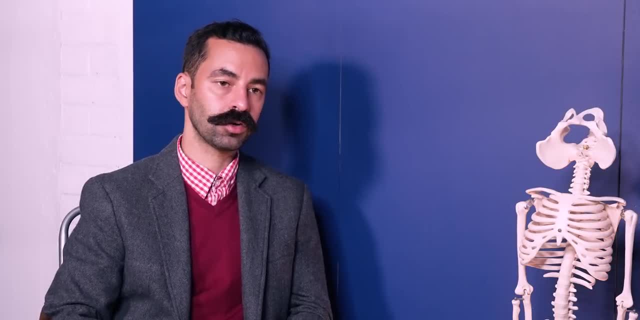 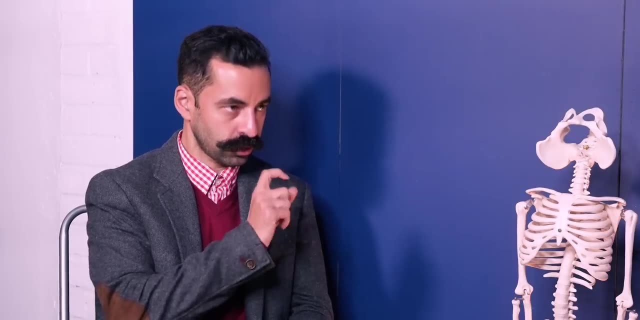 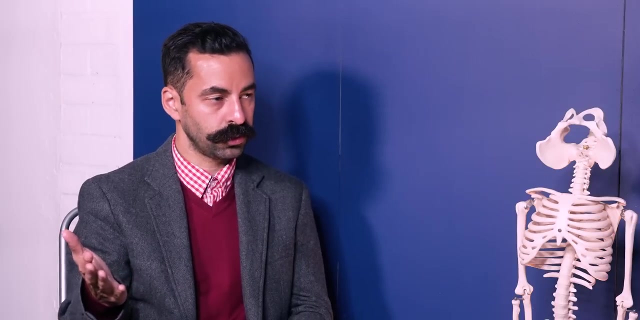 of true continuous blood pressure monitoring, Because to do that you need to have a line in your artery. There's non-invasive blood pressure, by definition, is just a snapshot because you have to do that whole inflation- deflation process. So the only way to truly measure continuous blood pressure- 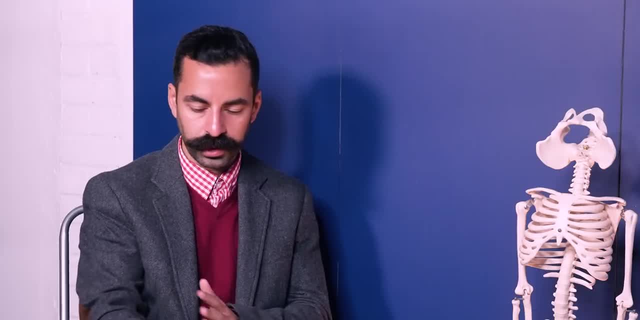 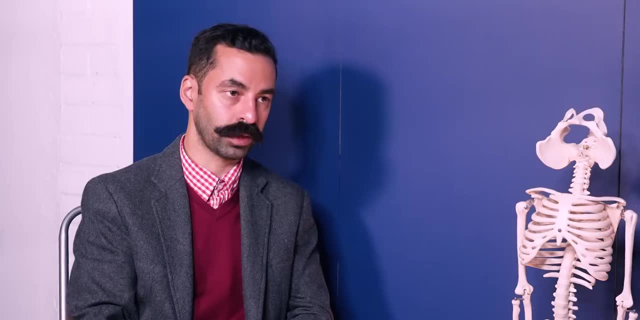 is by putting a line into an artery in the leg or the arm, And this is what I do when I do procedures, But obviously I'm doing that on patients who are sick And we have done short-term measurements of healthy volunteers but we have no data long-term. 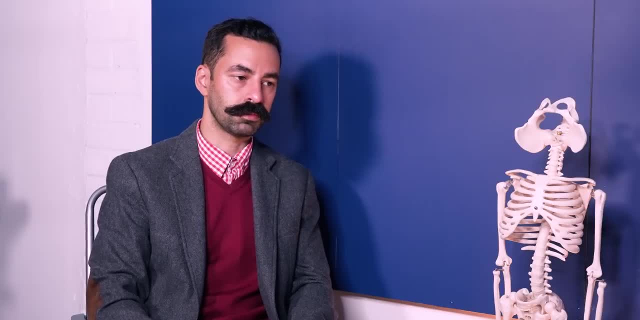 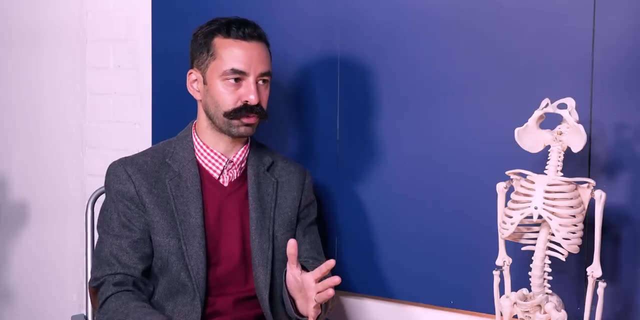 It would be completely unethical to expose somebody to the risks of having an invasive line in something that can just pop out and bleed profusely for any period of time, And especially during exercise. I don't want to be, you know, running along. 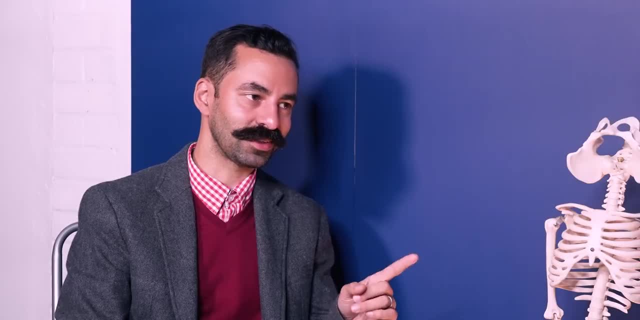 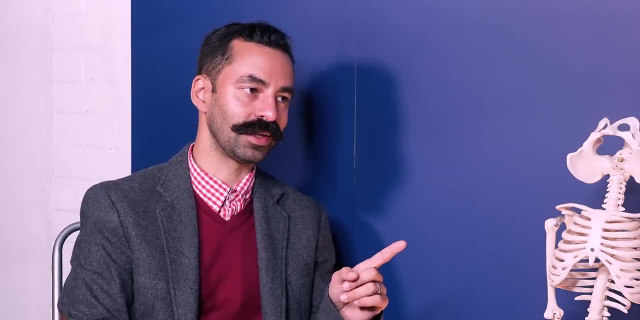 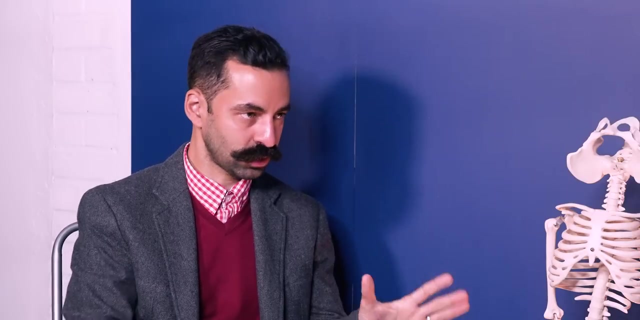 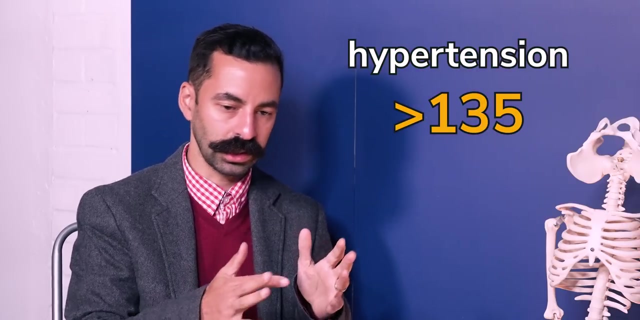 Now this is where reading the historical medical journals is always great fun. They put arterial lines in weightlifters and measured their blood pressure during a deadlift. Now, so we've said the definition of hypertension is more than 135, 140.. 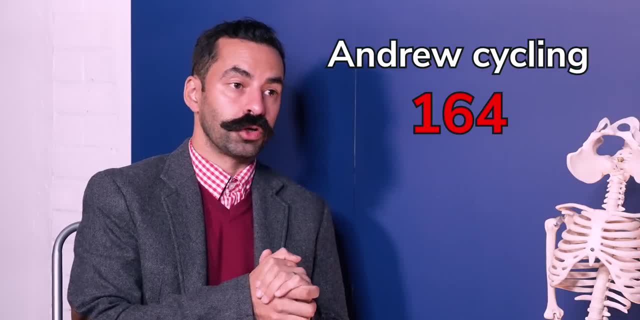 You got up to 160-something. A giraffe, Which we Think is, you know, the highest blood pressure in the animal kingdom. I mean, it's got to get the blood all the way out to the top of the head, presumably. 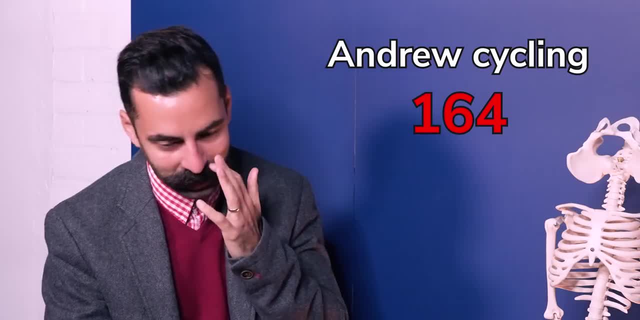 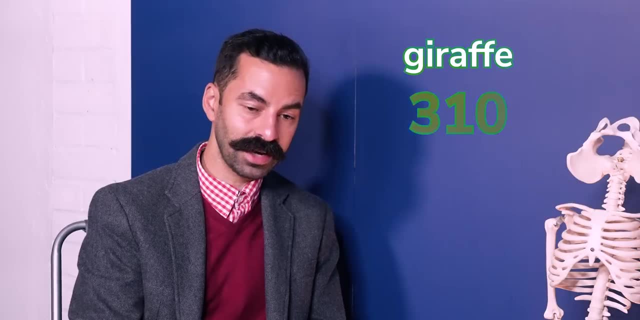 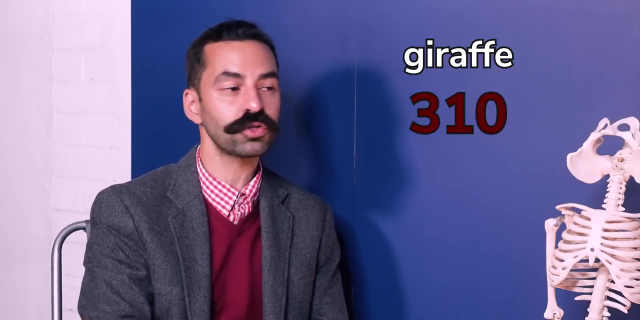 Exactly So we've. I love these papers. you know where they've measured giraffe blood pressure. I think it was about 310. systolic was a giraffe blood pressure. What do you think the blood pressure recorded in a weight lifter doing a deadlift was? 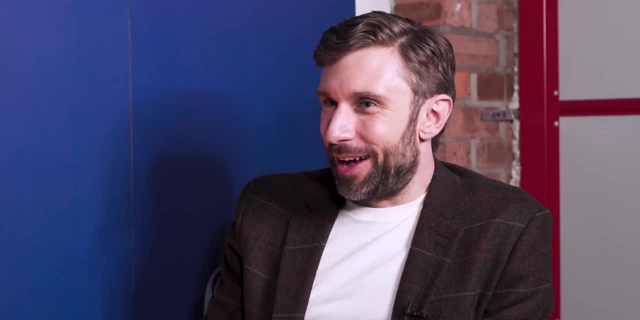 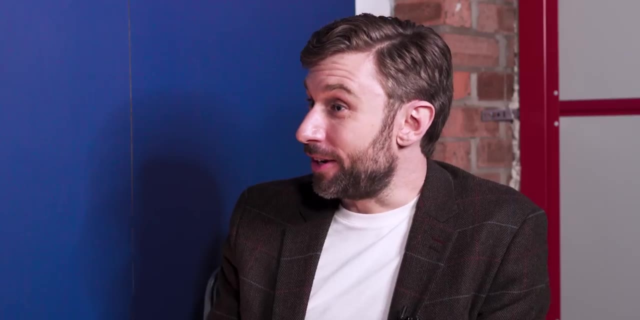 Transiently, you know, just for the deadlift, I'm going to say 400.. Yeah, it was over 400.. Wow, 435,. I think That's incredible And you can imagine it like watching their veins strain. 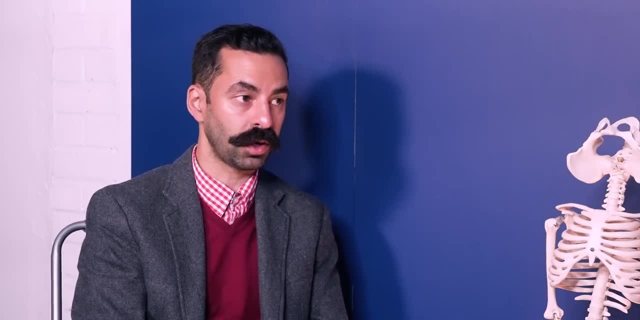 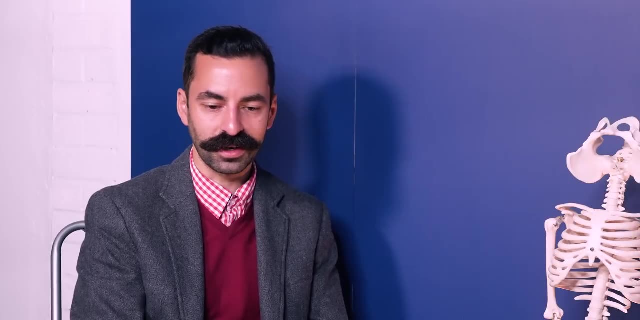 Well, I mean, there are lots of videos online of deadlifters. you know just passing out after. So you know I wouldn't advise Eddie Hall deadlifting a car kind of level. but weight training is good, You just don't have to go crazy. 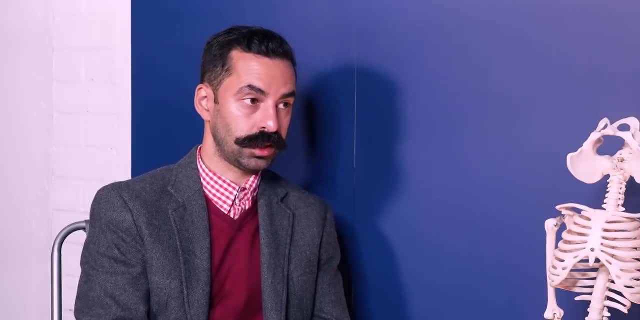 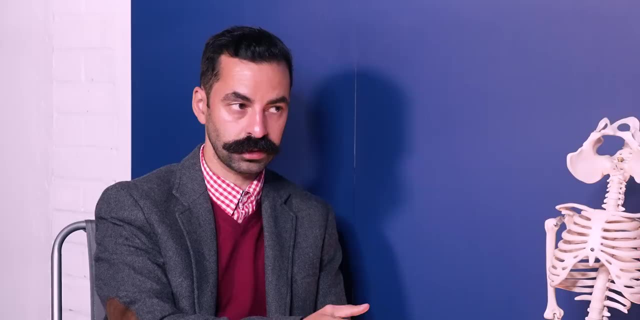 So, yes, the body can handle short term. you know spikes like that, I think at that Extent you can do a lot of damage. but you're you measuring 160 during exercise? That's nothing to worry about at all. And also- this is one of the nice things about exercise and blood pressure- is immediately you can see the benefit. Some of the benefits of exercise take a bit longer, but blood pressure while it'll spike, like in your case, straight away after you get a drop in blood pressure. 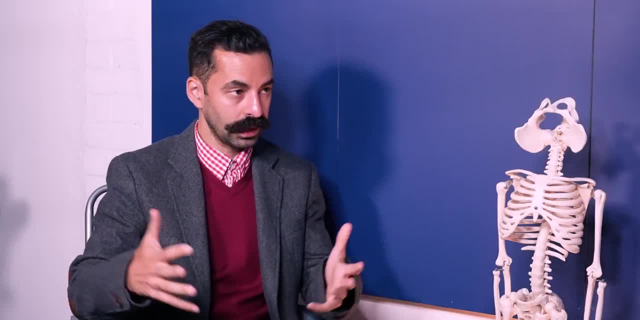 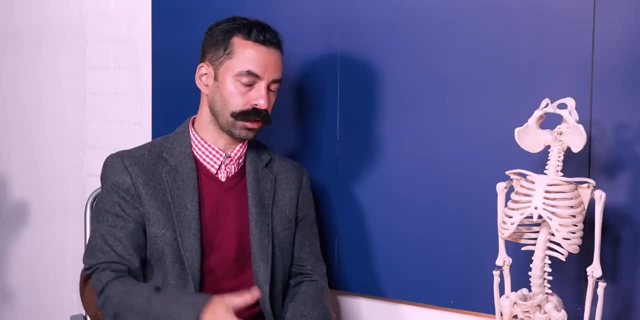 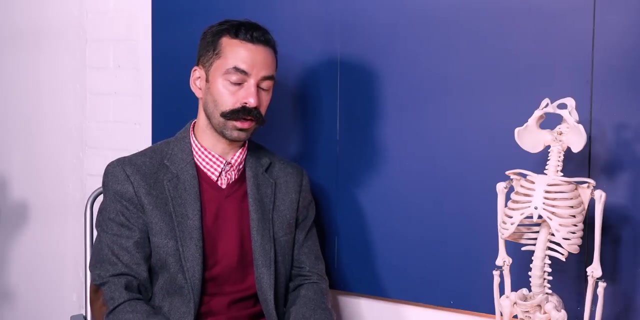 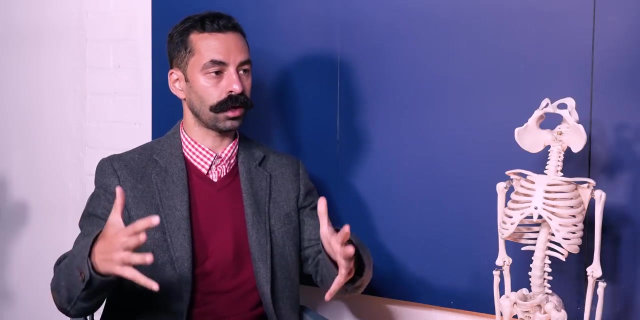 And this is because you've got a release of nitric oxide in the body, which is this chemical that opens up your blood vessels, and we administer nitrates in patients who have circulation problems, But you can have your own endogenous supply And so you get an immediate benefit, post exercise, of all your blood vessels having opened up. 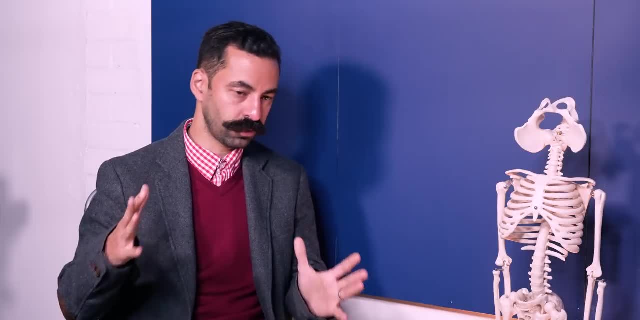 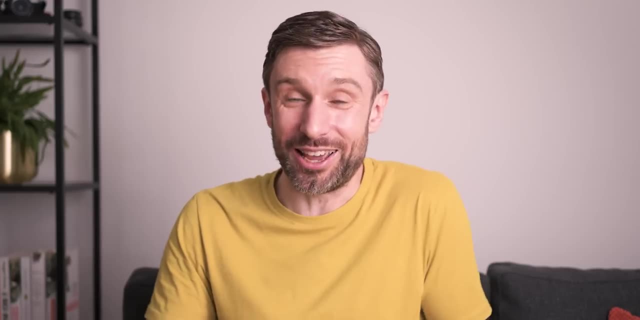 and a nice drop in blood pressure, which is why it is one of the most important treatments for high blood pressure. So this is one case where it's totally OK to get high on your own supply or get low, Since we're talking about blood pressure, I guess 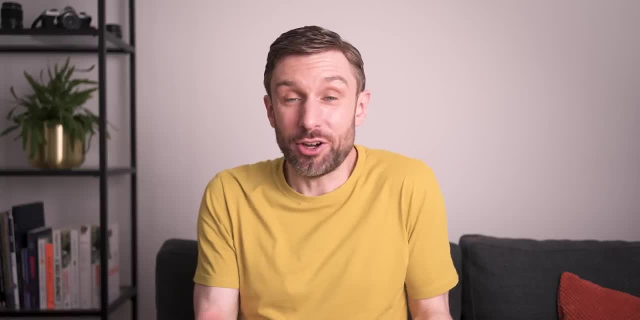 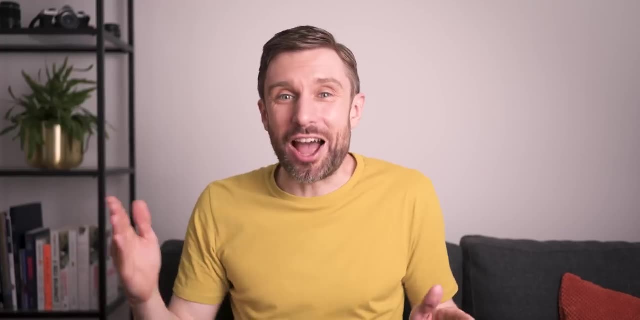 So blood pressure is an absolute classic medical measurement used by doctors for decades and with loads of high quality evidence telling us how important it can be for your health. So now we're going to move straight to the other end of the fitness data fashion spectrum and look at an up and coming new kid on the block when it comes to health monitoring: heart. 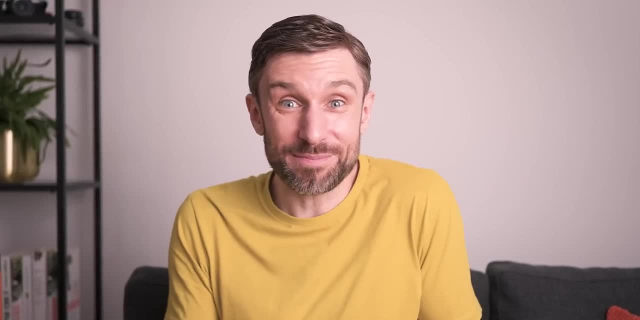 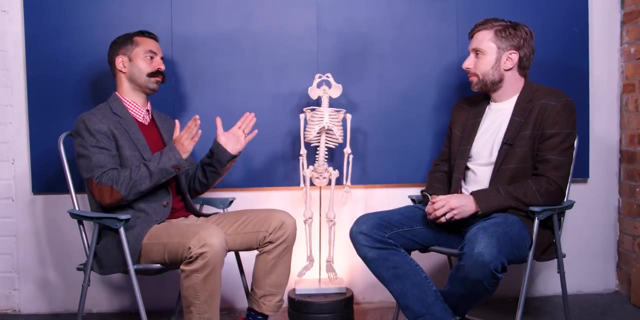 rate variability, or HRV. So what is it and why is it important? Put simply, heart rate variability is the variation, put simply, in the gap between heartbeats. So you might think that the heart just sort of beats like a metronome. 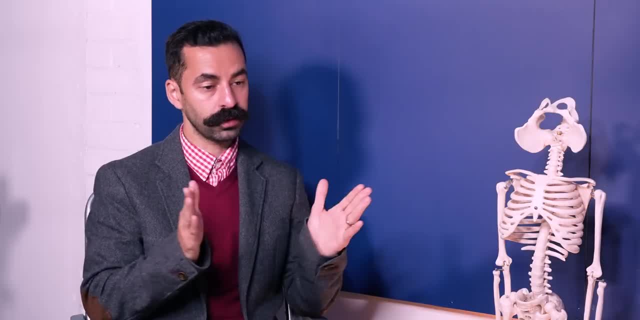 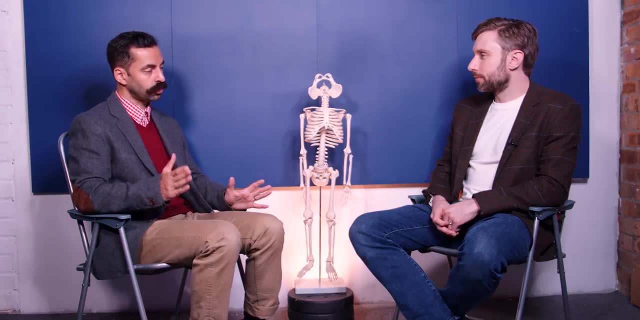 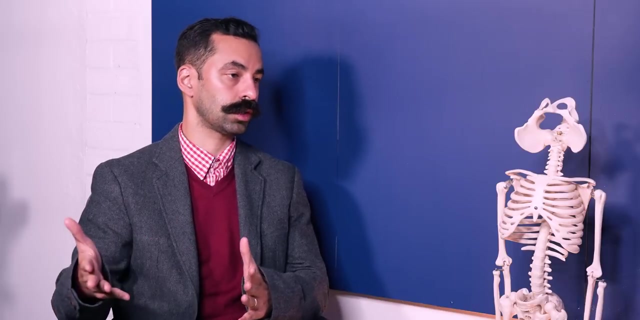 constantly. but actually in a healthy heart you get this slight variation in the gap between each heartbeat. It seems counterintuitive but you might think a regular heartbeat is good. but actually a variation seems to have a prognostic benefit. so it seems to be a. 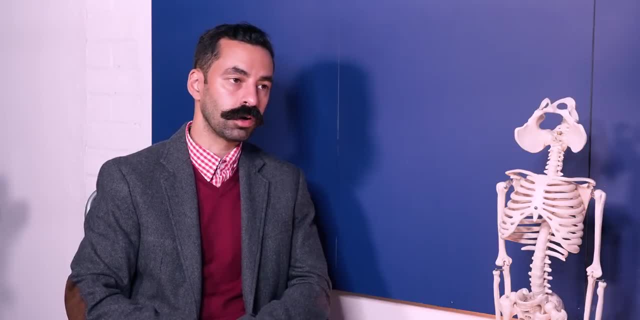 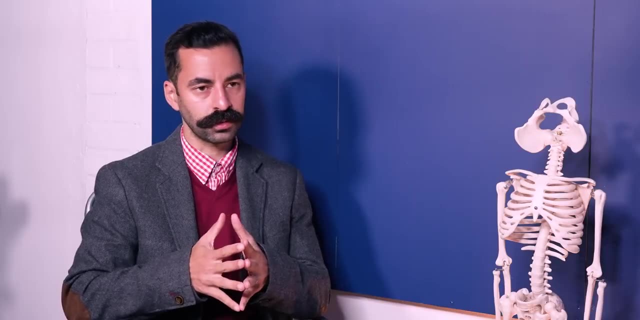 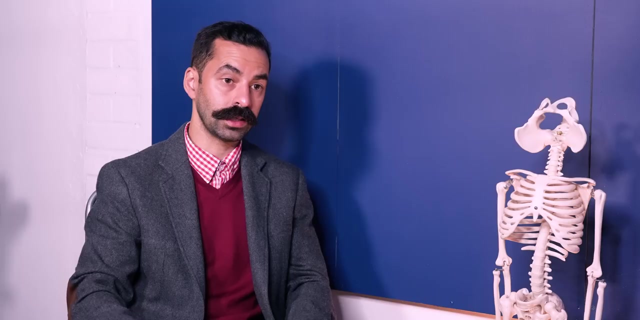 marker of good health, And this came out of continuous heart rate recordings after patients had had heart attacks- and this, I think, is going back way into the 70s or 80s- and it was found that the heart rate variability decreased and these patients did worse. And then the same thing. 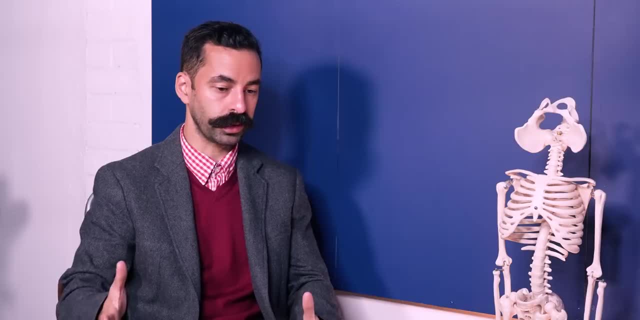 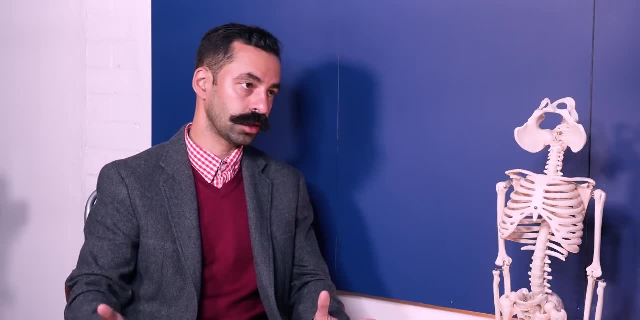 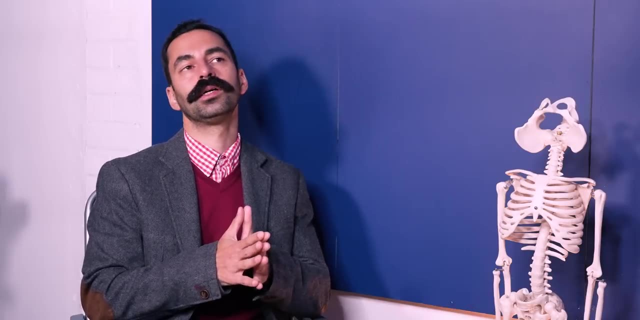 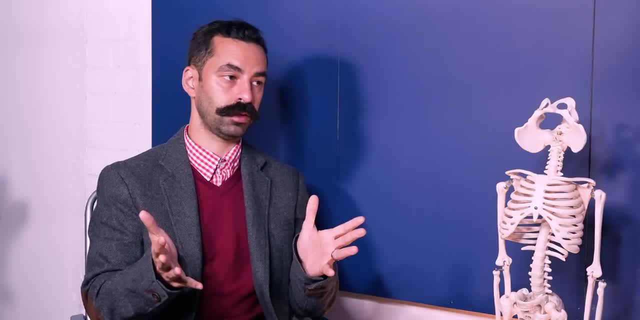 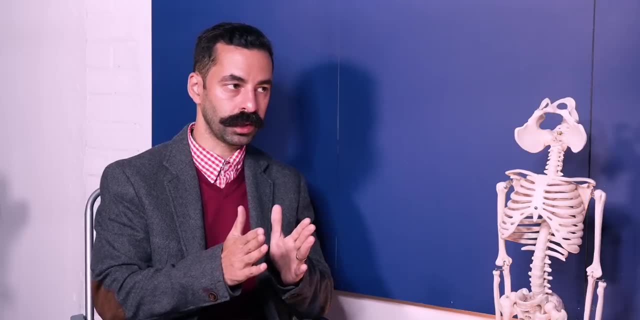 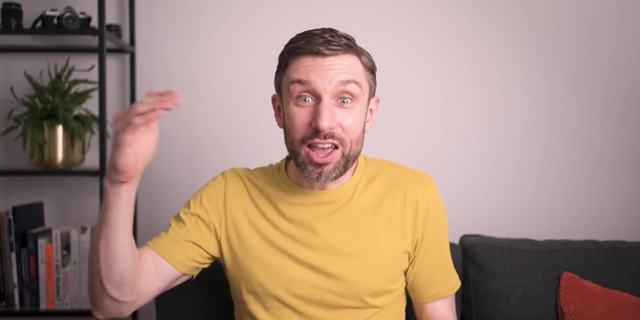 a marker in non-pathological states. So if you don't have any of these diseases and you're just healthy, whether tracking your heart rate variability is something you should be doing, The best slightly hand-waving explanation I've heard as to why higher variability is good is because it shows 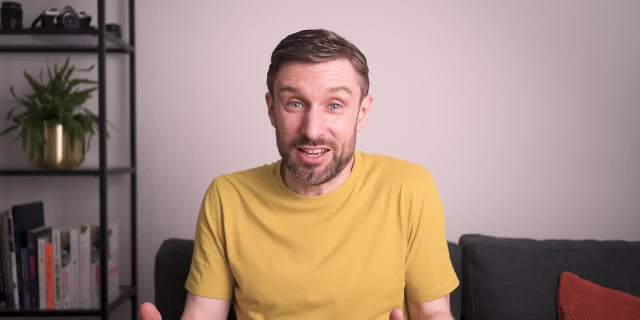 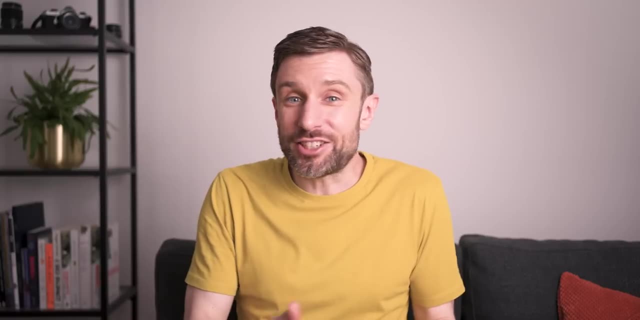 that your heart is highly adaptable to changing circumstances, rather than being in a stressed out non-adaptable state, And this could plausibly be important for your health, because your heart rate needs to change all the time for loads of different reasons, as your activity level varies throughout. 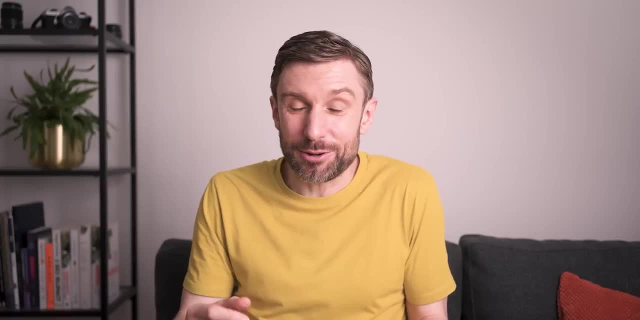 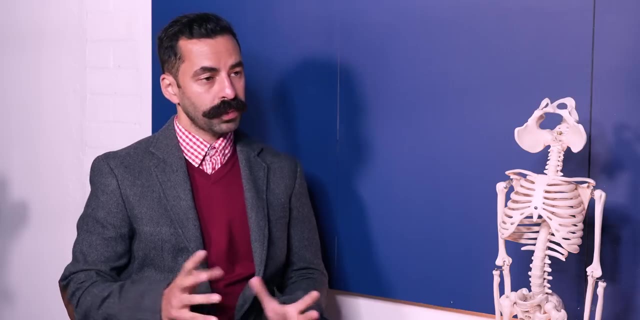 the day, Your heart rate even changes slightly depending on whether you're breathing in or breathing out. So clearly that ability to adapt to changing circumstances could be pretty important. One application that I've heard is that the heart rate changes slightly depending on whether you're. 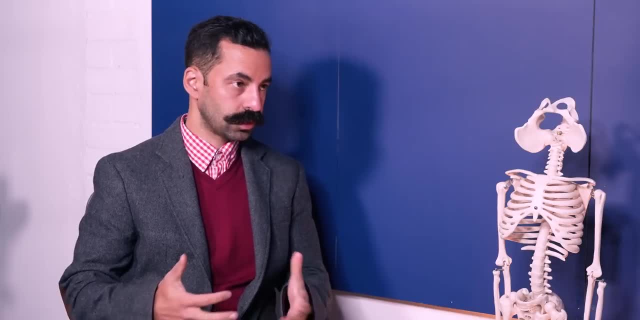 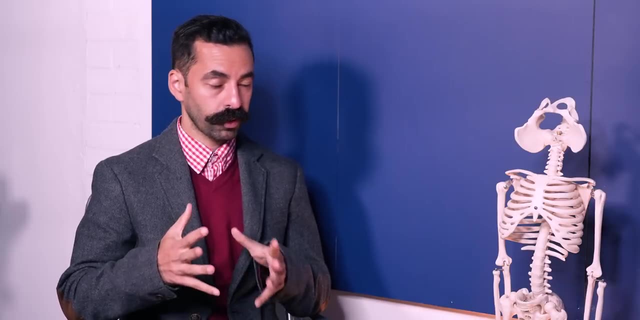 breathing in or breathing out, So if your heart rate changes slightly depending on whether you're breathing in or breathing out. Another application of heart rate variability which is of interest to, I think, a lot of athletes- and it seems to be picking up in its popularity- is using heart rate variability less as a sort of 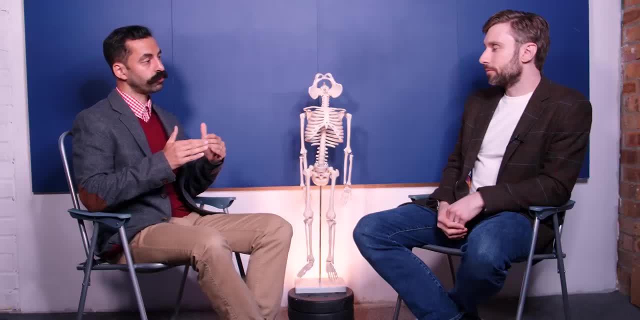 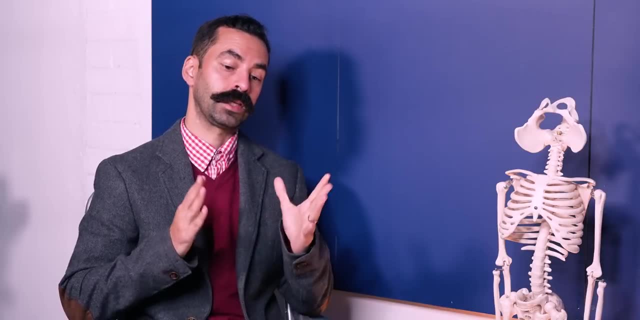 long-term thing to track but also to inform regarding recovery. This is where we start crossing into it A little bit of hocus-pocus, But heart rate variability, can you know? different devices will have different ways of doing it, but they typically will say: 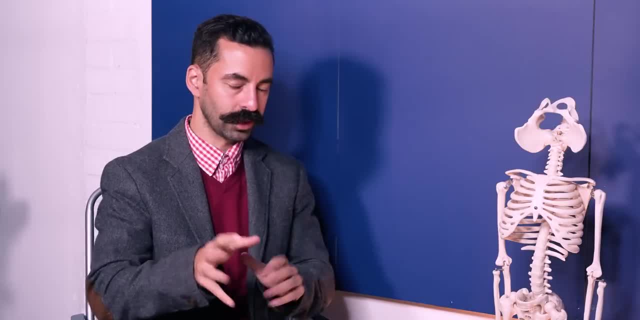 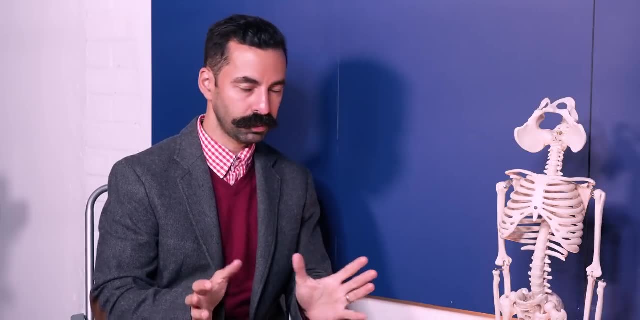 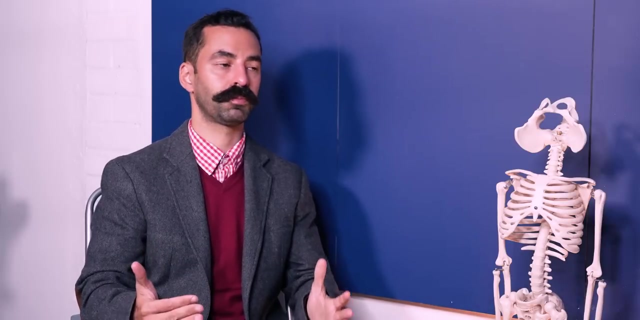 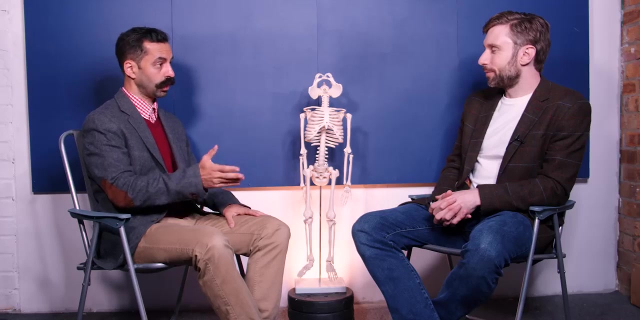 bad, medium, good kind of ranking, And if your heart rate variability is good, suggesting you've had a good sleep and you are in a good state to be doing something strenuous because your powers of recovery will be good. And then I've often heard people say: oh, you know, I looked at my device and it said that my HRV was in the 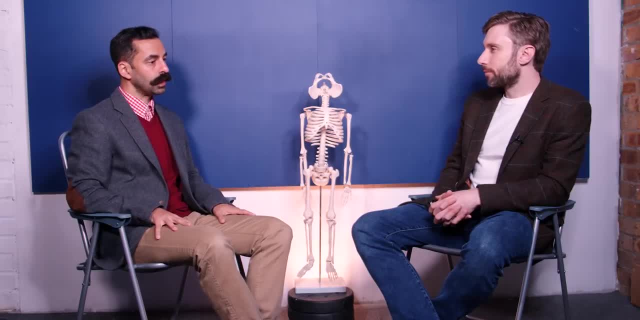 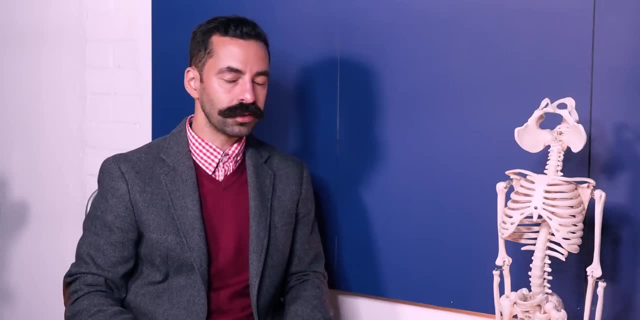 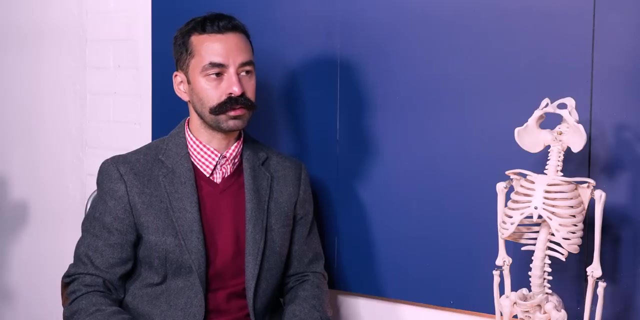 red zone today, so I'm not going to do any exercise and this was reflective of, you know, my, my sleep pattern last night and I'm like, okay, that's fine, But you know, if I've had a bad sleep, I gotta know I've had a bad sleep. I don't know if I need a heart rate variability to tell me that. 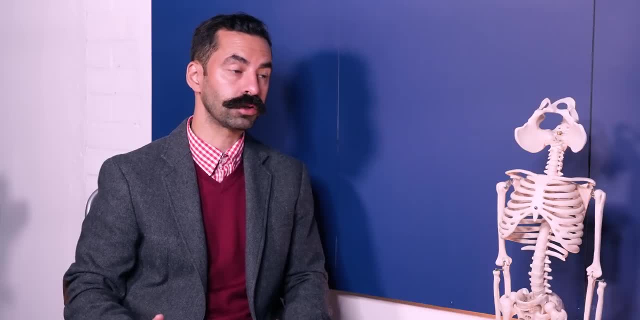 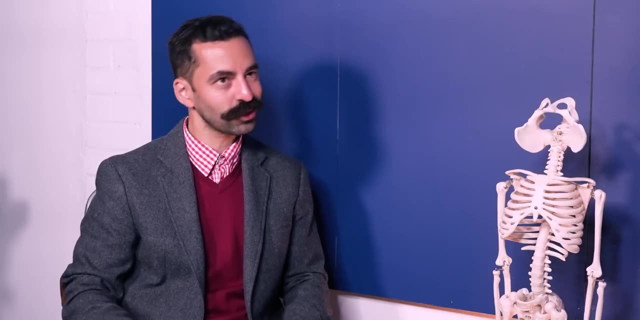 And other people have said. well, I noticed my heart rate variability and my sleep quality really deteriorate when I've had a few drinks before bed. I'm like, yeah, I think I could have told you that that as well. you know, like i don't know, that we, i think i feel like we sometimes over medicalize. 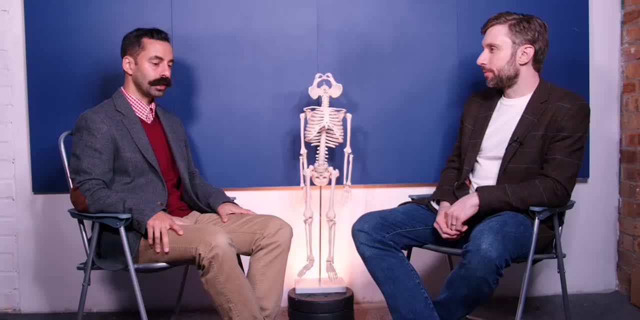 some of just common intuition, common sense things, um. but yes, there seems to be uh interest in sporting circles and that clearly inevitably crosses into more general wellness. but i would always take anything that elite athletes do for their health with not just a pinch but a shovel of salt. it's gonna be terrible for your blood pressure. blood pressure, since getting a smart